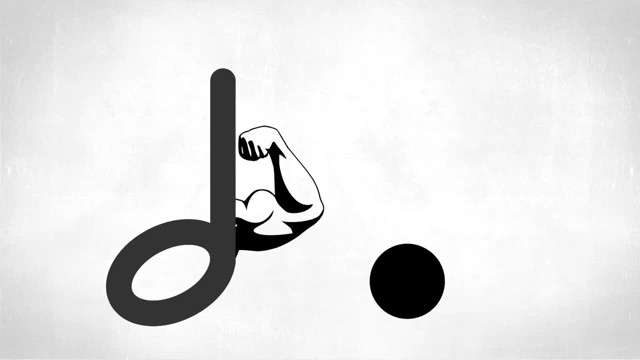 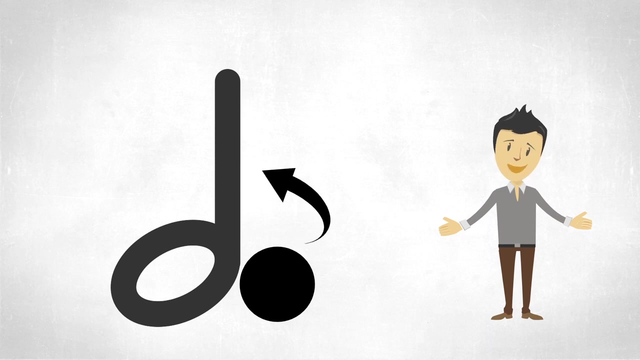 Think of a dot as a little brother to the half note. He wants to hang out with the half note but is smaller and doesn't get as many beats as the half note. The dot is actually only ever half of the value of the note he sits next to. Okay, let's break this down. Francis looks at his big 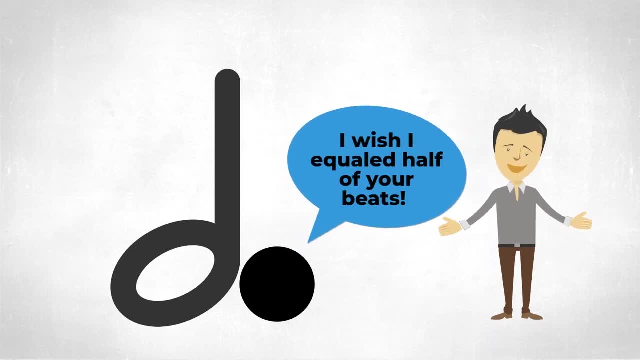 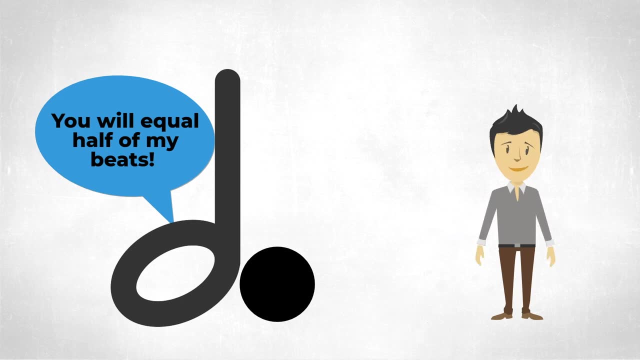 brother, halfy the half note and says, oh, halfy the half note. I wish I equaled half of your half. Well, says, halfy the half note, since you're hanging out with me, you will equal half of my. 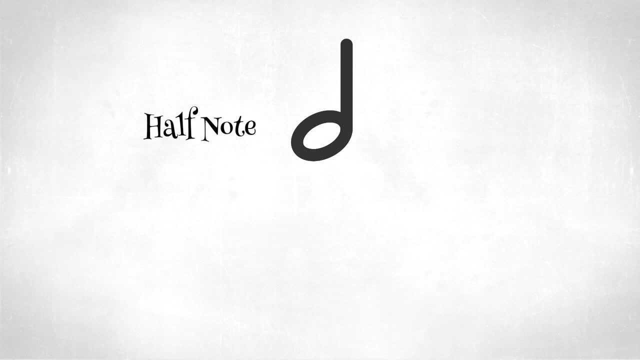 beats. The dot was pretty excited to hear that, Since the half note equals two beats, we will need half of two, which is one beat. So the dot equals one beat. when sitting next to the half note and when we add the dot, we also add one beat. Put them all together and the half note with 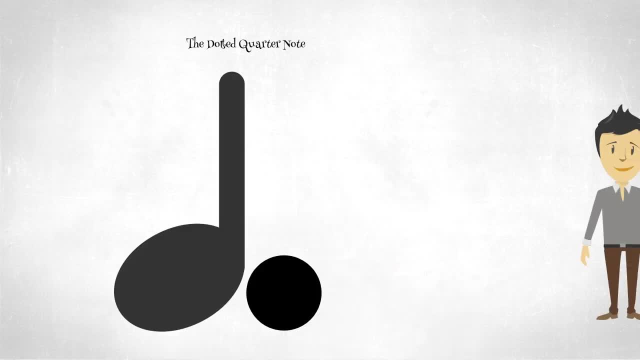 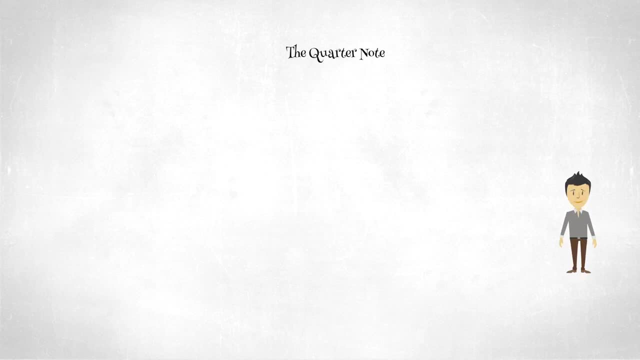 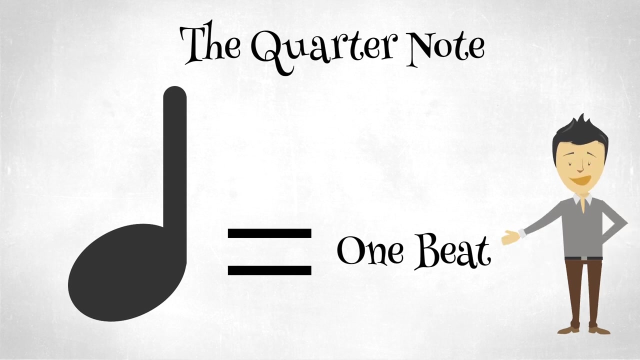 a dot equals three beats. The dotted quarter note is similar to the dotted half note. Wow, Remember, the quarter note equals one beat And, of course, the dot can be connected to the quarter note. Oh, here he comes again. Hey, Francis. 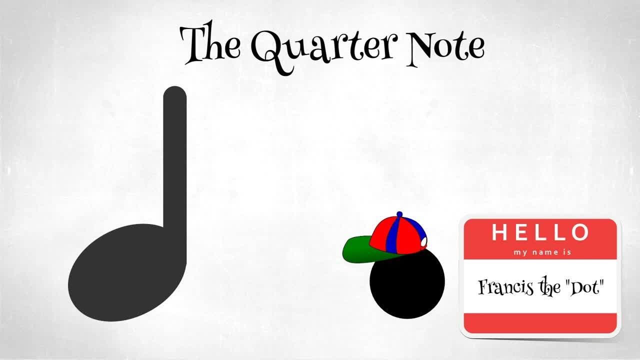 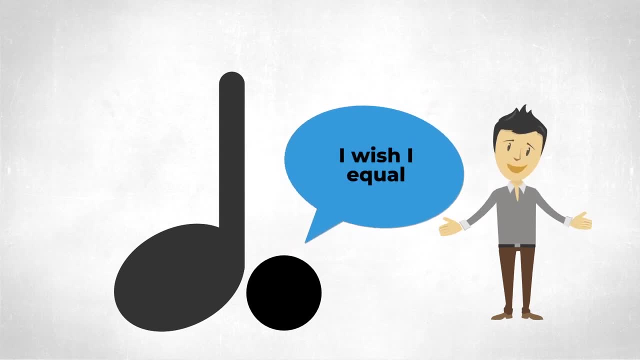 Francis will look at the quarter note and say the same thing. I wish I could say the same thing. I wish I equaled half of your beats. And the quarter note will say the same thing. You know, since you're hanging out with me, you will equal half of my beats. 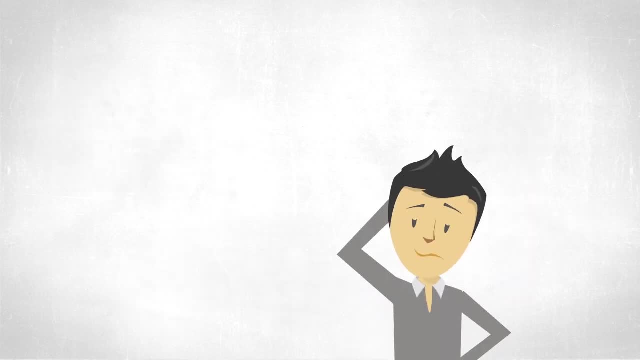 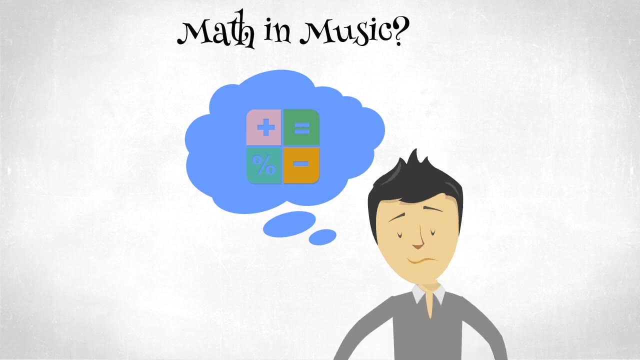 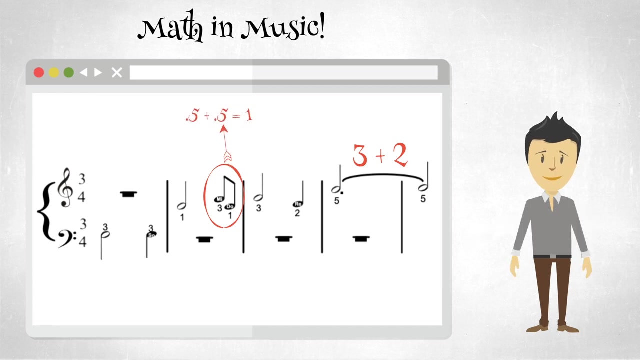 Yeah, Okay, Huh. This is where things can get a little complicated. We need to do some serious math here. Math and music. Whoa Yes, Math is found all over the place. Five and music. 0.5, just 0.5 equals five. 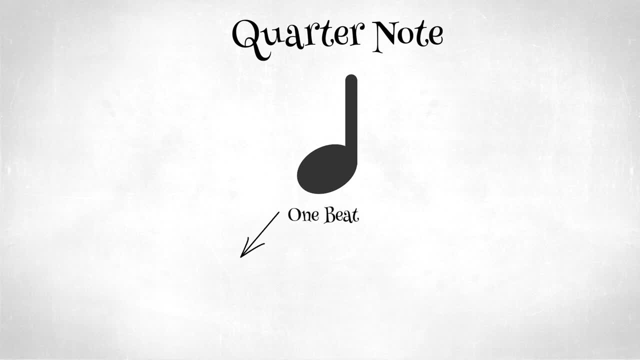 So the quarter note equals one beat. If we take one beat and split it in half, that means you would have two single eighth notes. Single eighth notes only equal half of a beat. So if you add them together they would equal the same as a quarter note, because half plus.